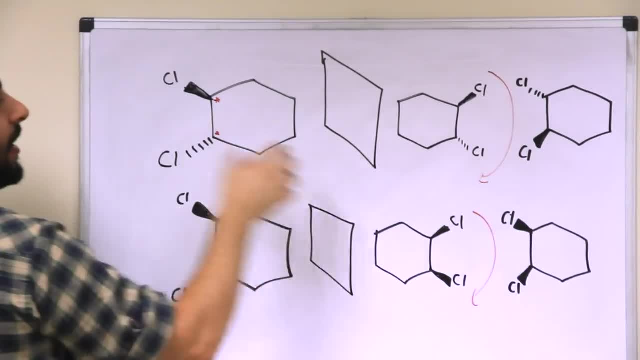 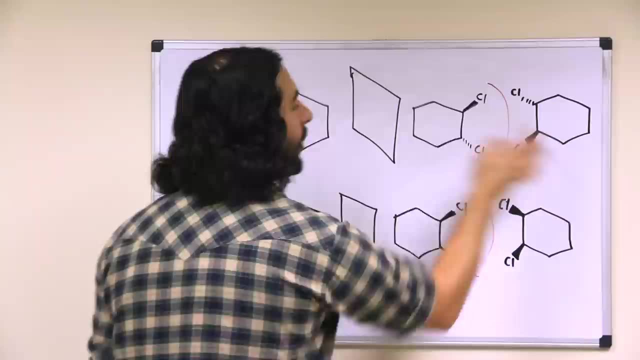 going to see that it is not going to work. this is not going to fit because a dash chlorine will be on a wedge and a wedge chlorine will be on a dash. Therefore, these are non superposable mirror images. they are enantiomers, one of one. 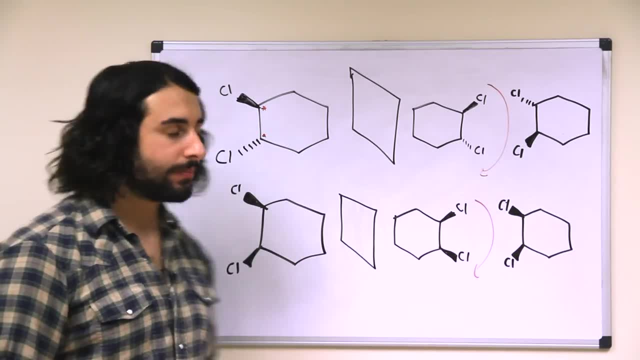 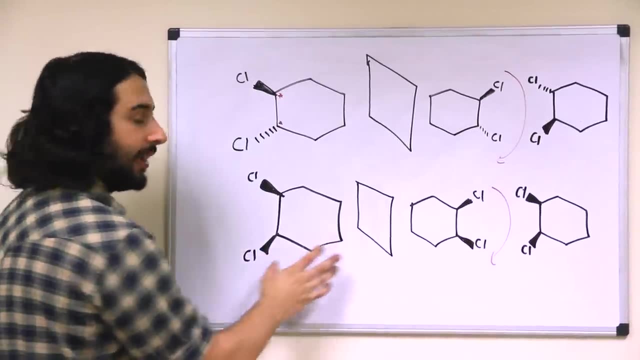 another. therefore, this molecule is chiral. but what if we do something as simple as just changing this dash to this wedge? now what we're going to see is, if we reflect across the mirror plane, this is what we're going to get. we turn this a 180 degrees and we're going to see that the whole board is 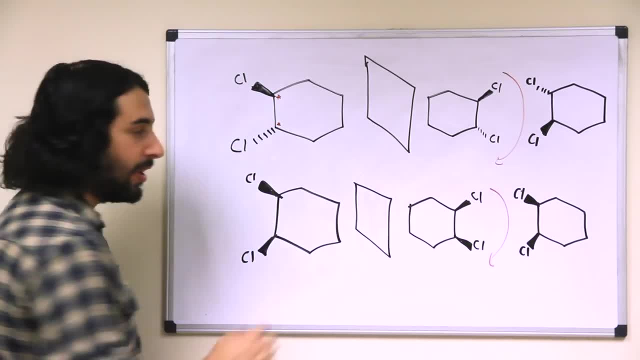 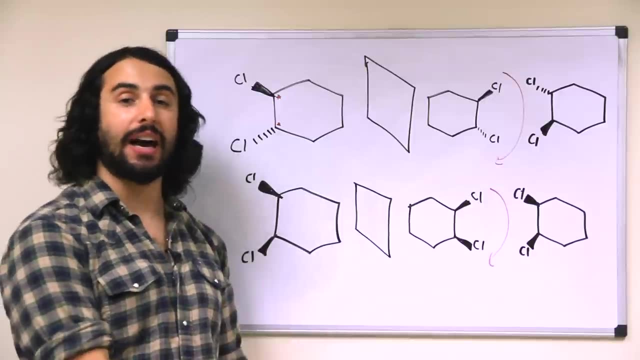 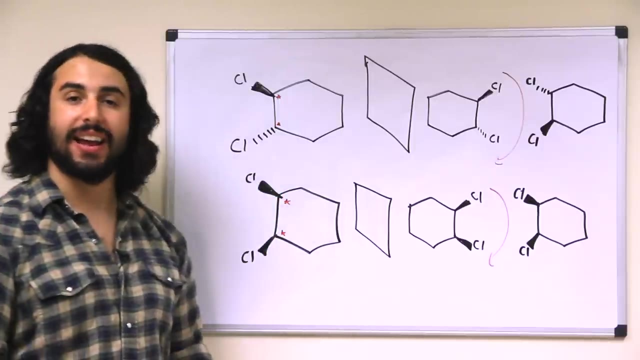 we find that this is flawlessly superposable, so the mirror image is identical to the original. therefore, by definition, this is achiral or not chiral. however, it does still have two chiral centers and you ought to be able to assign absolute configuration to these two chiral. 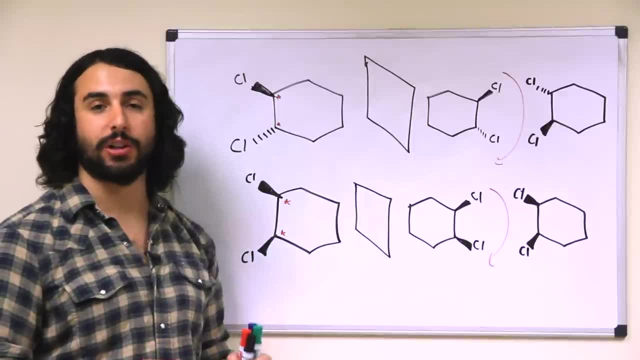 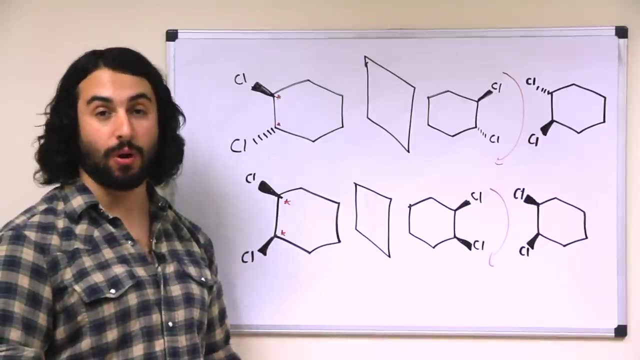 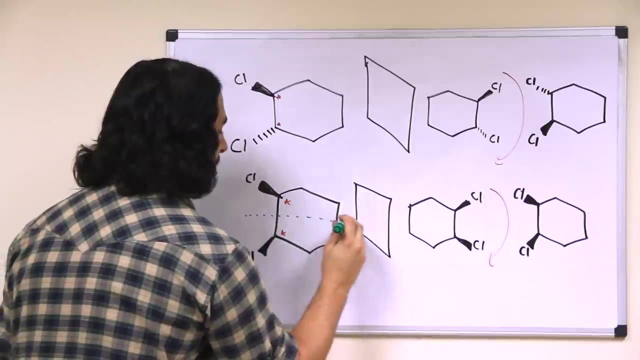 centers. so this means that it can be possible for a molecule to have two or more chiral centers with their own absolute configurations, but be achiral overall. and in fact there are special terms to designate why. and in this case it is because this is something called a mesocompound, a mesocompound. 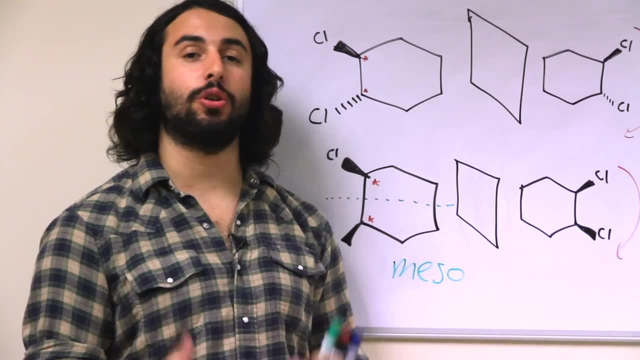 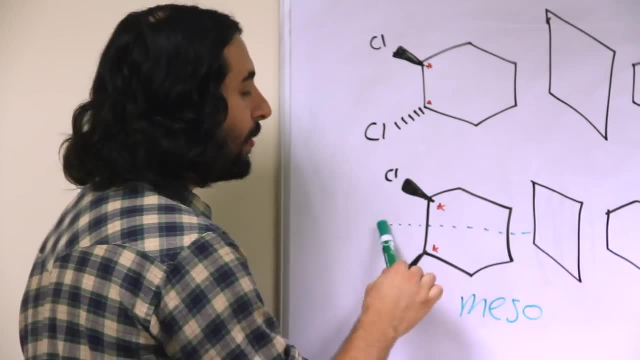 is a compound that has an internal plane of symmetry. what that means is because the top half of this molecule, when reflected across this central line of this central line of this molecule, when reflected across this central line of this central line of this molecule, when reflected across this central line of 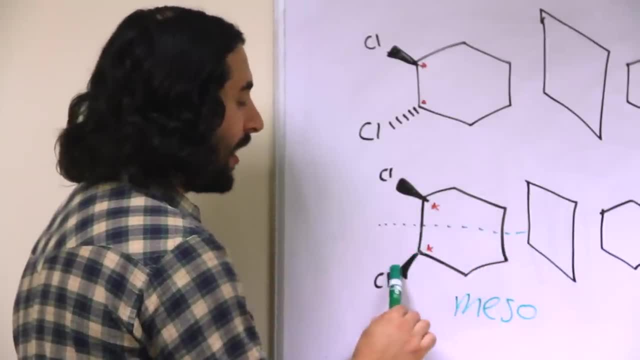 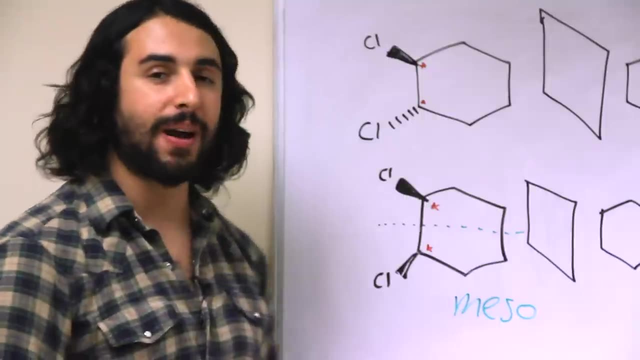 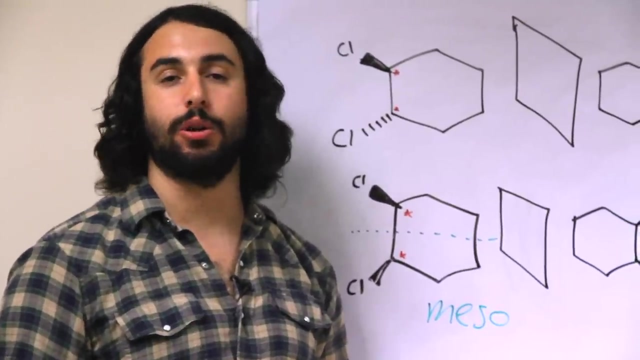 plane does in fact give accurately the other half of the molecule. that means that this is a plane of symmetry. therefore it is a mesocompound and any mesocompound is achiral or not chiral. so if you want to see whether a molecule with two or more chiral centers is chiral overall or not, 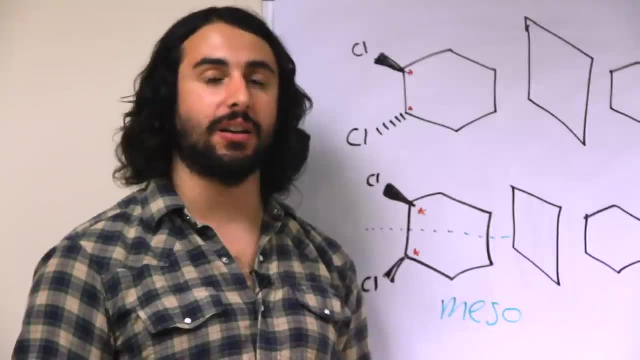 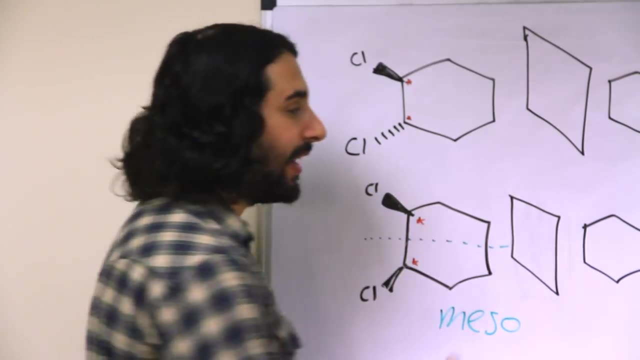 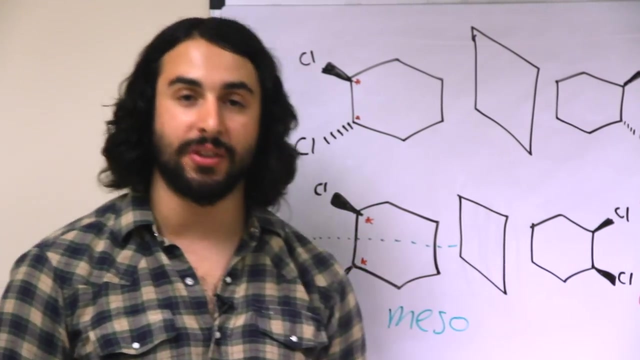 you can either examine for any kind of planes of symmetry or, as always, you can simply go ahead and reflect across the mirror plane, see what you get and then investigate as to whether the result can be superposable on the original. so there's another kind of internal symmetry that. 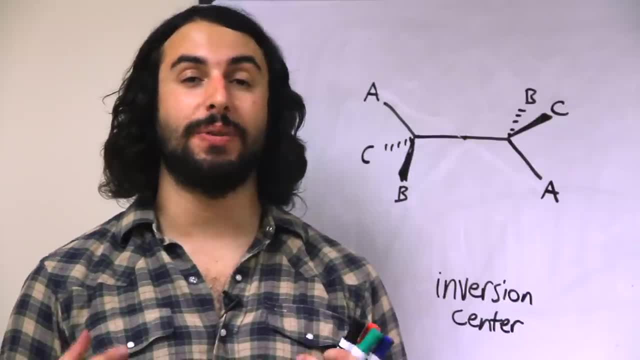 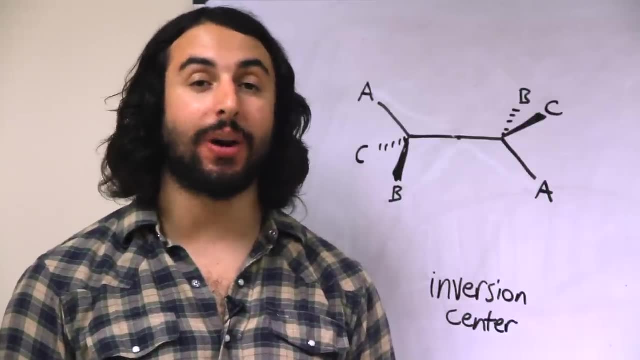 will allow for a molecule with multiple chiral centers to be achiral. overall. it's a little bit different from mesocompound, because it's not a plane of symmetry. it's actually more like a point of symmetry called an inversion center. so let's take a look at what this is doing. so, if you reflect, 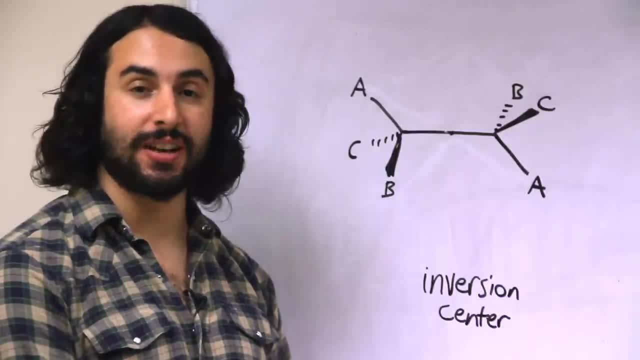 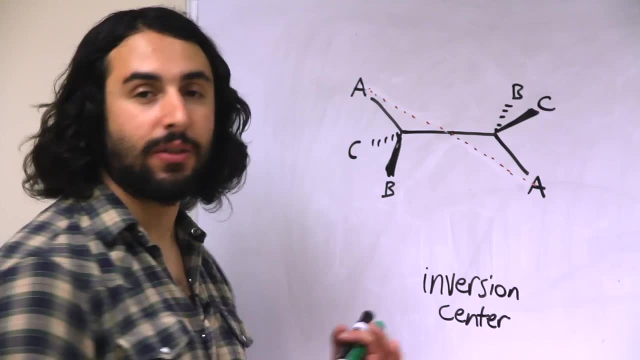 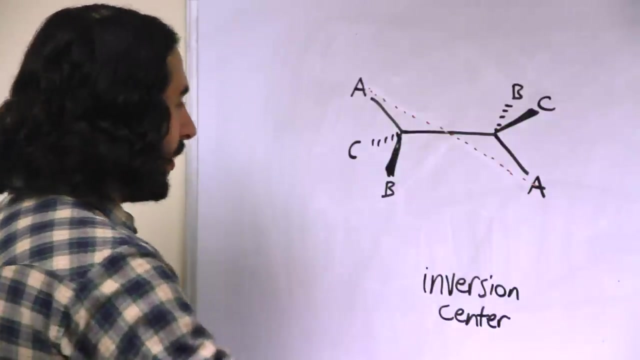 every atom in the molecule across the inversion center at the center of the molecule. this is what happens. so A will see A on the other side of the molecule. those are both in the plane of the board. now B here is extending out of the board and that is going to go through the center to the dashed B. 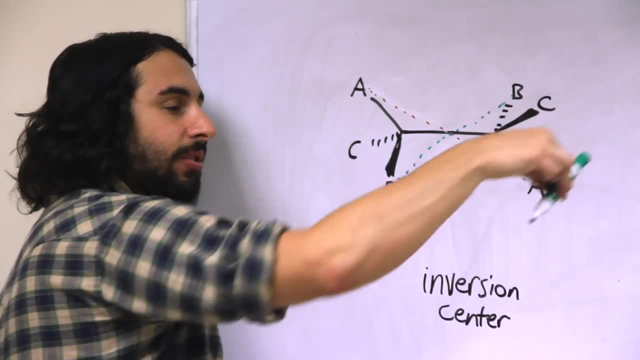 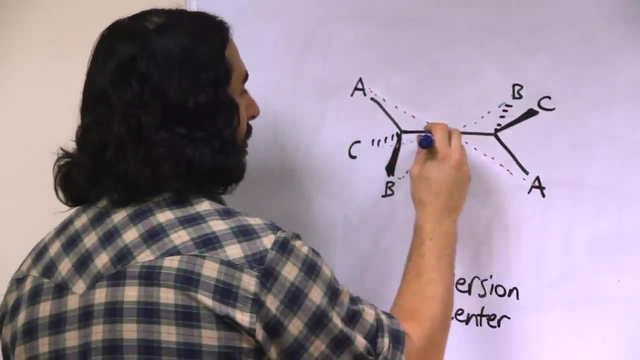 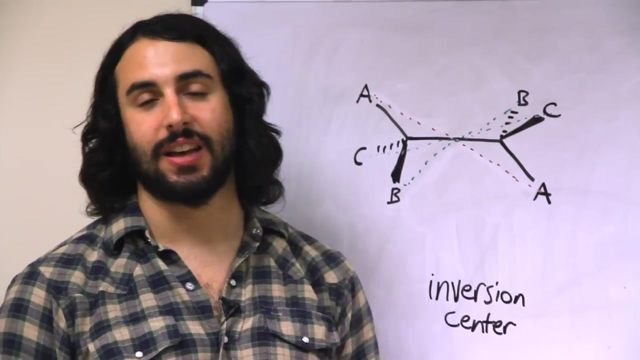 on the other side. so that's passing through the center and through the board onto the other side and then likewise the C that is coming from the other side past the board will travel through the center and then to the C on the wedge over here. so if it is the case that every atom in the molecule can be reflected across an 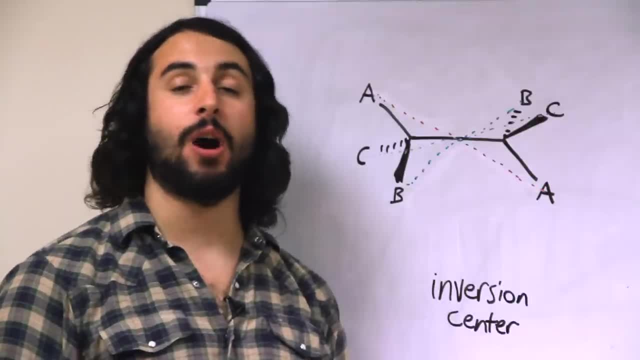 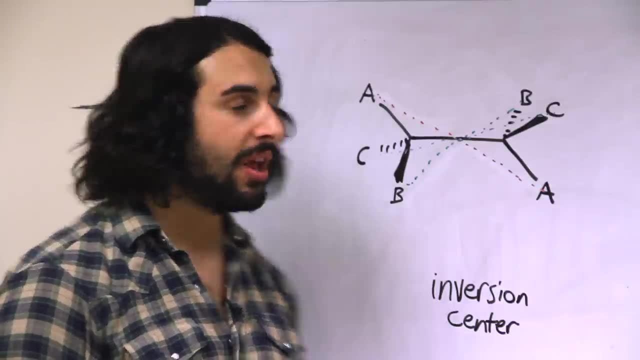 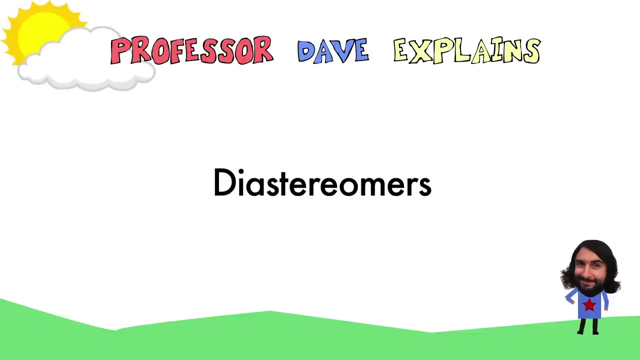 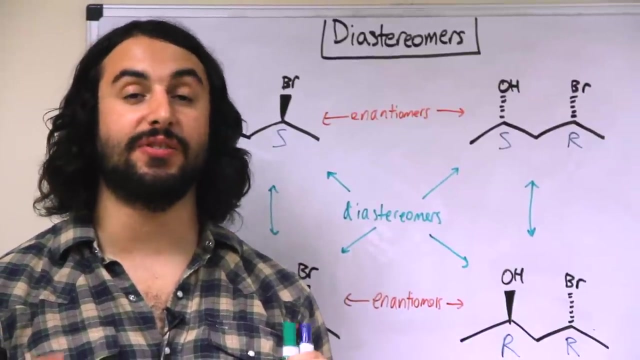 inversion center and see itself on the other side. that molecule has an inversion center and is therefore achiral overall or not chiral, even though there could be, just as in this case, two chiral centers. so there's another stereoisomeric relationship that we need to be aware of, and that is that of 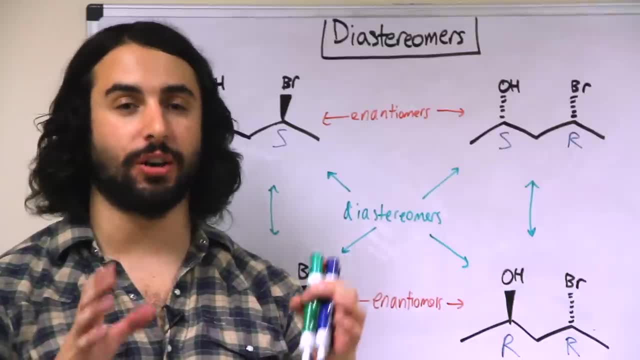 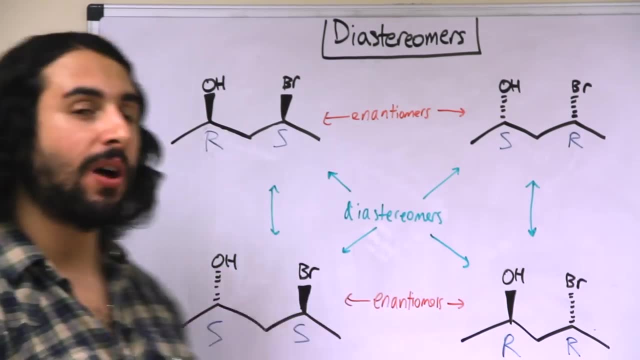 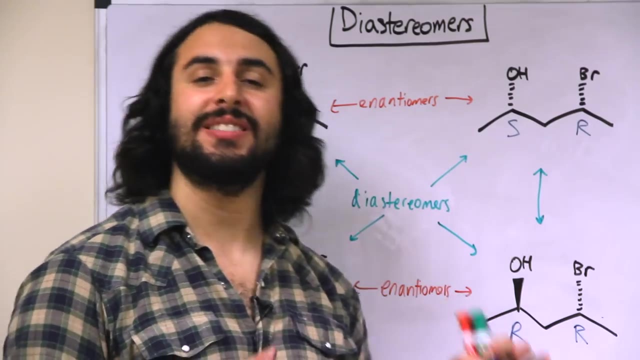 diastereomers. diastereomers are stereoisomers that are not specifically enantiomers. in other words, they are molecules that are stereoisomers of one another, but they're not specifically mirror images of each other. so let's take a look at a molecule that has two chiral centers. 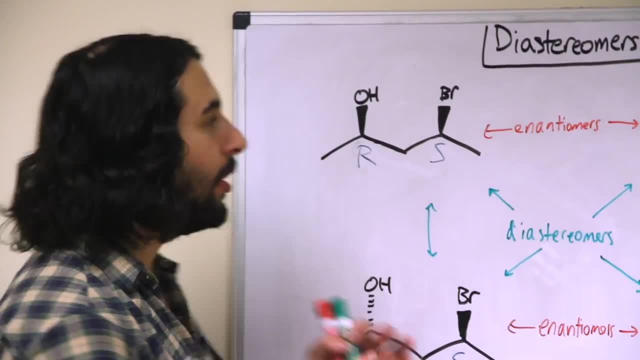 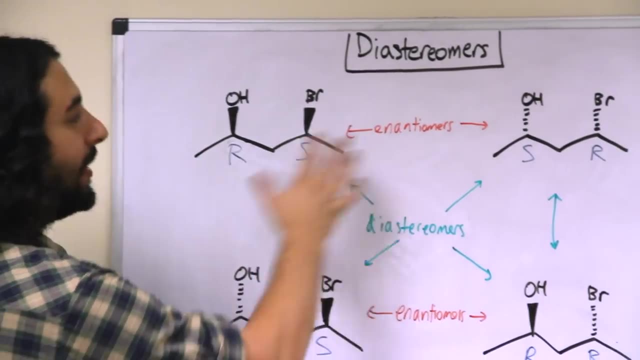 so here we have an R and we have an S. now we know very well that if we take the mirror image of that, that we're going to get the enantiomer. so that would be this and at home, if you want, you can go. 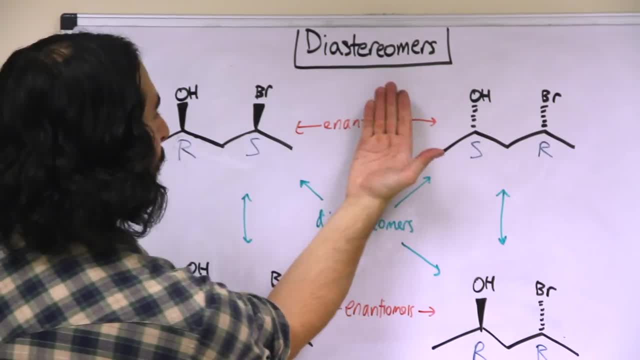 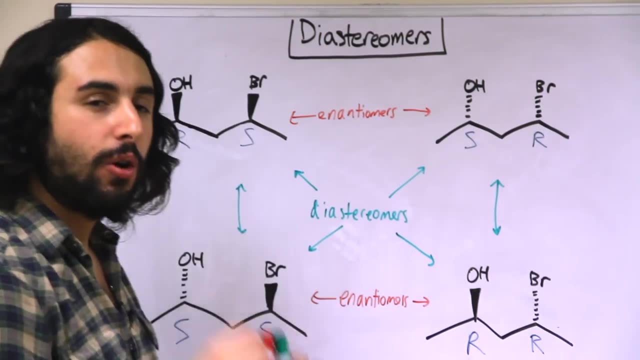 ahead and draw this across the mirror plane and then flip it over and you will see that you would get the same groups, but now those would be on the dash bonds. when you take the mirror image of something, or if you're drawing the enantiomer of a molecule, it is essentially the enantiomer of a molecule. it is essentially the. 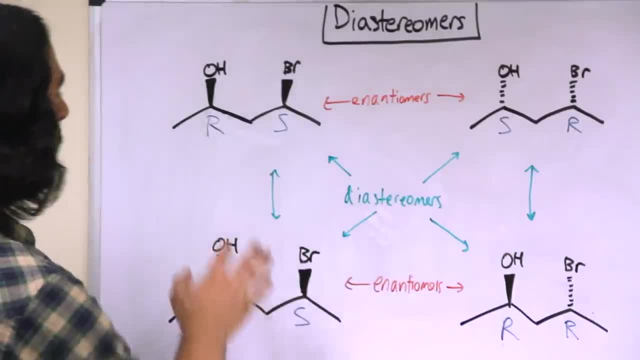 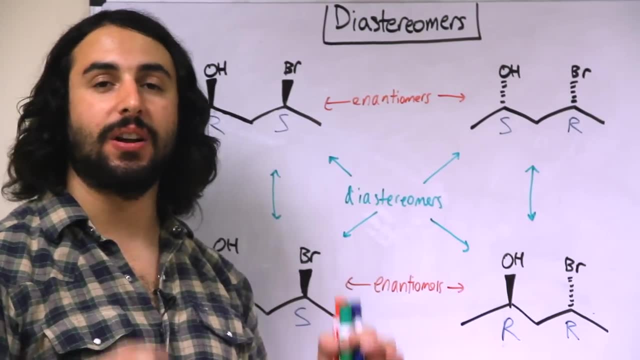 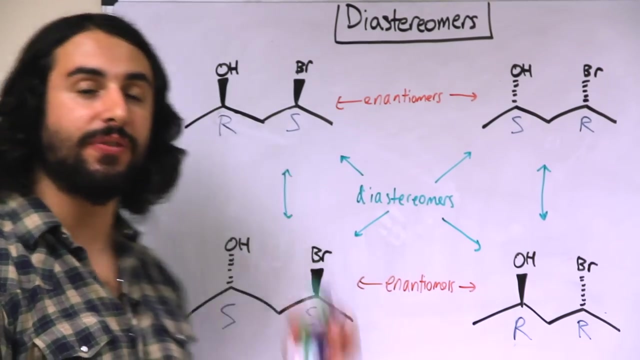 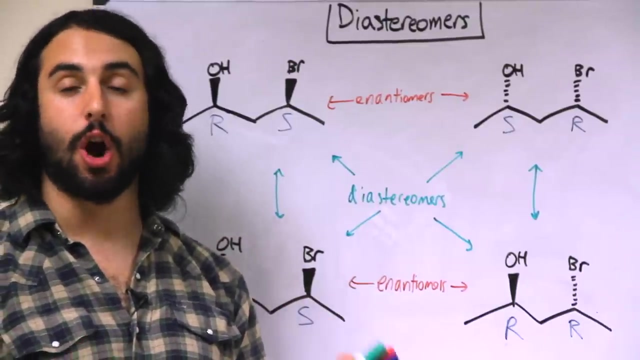 inversion of every stereocenter. so whereas this is R and S, this is S and R. so these are enantiomers, because they have precisely the inversion of each chiral center. now, a diastereomer of this molecule would be one in which one, but not both, of the stereocenters are inverted, so down. 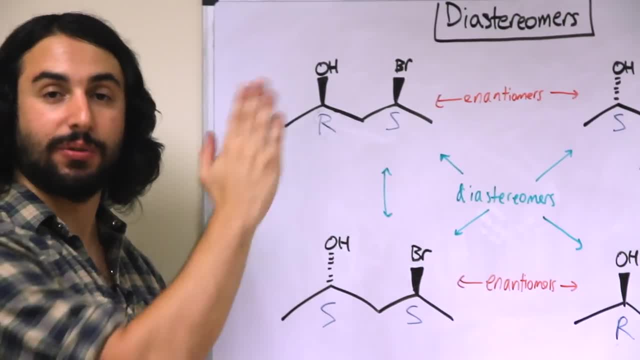 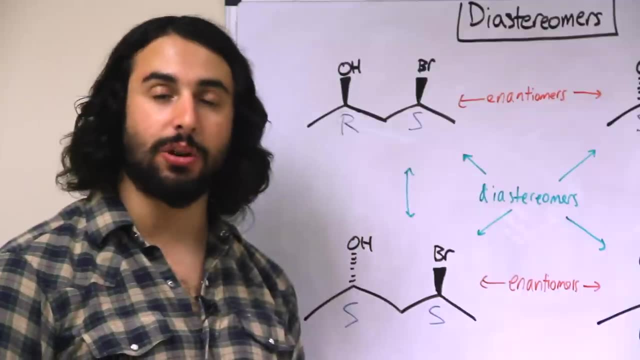 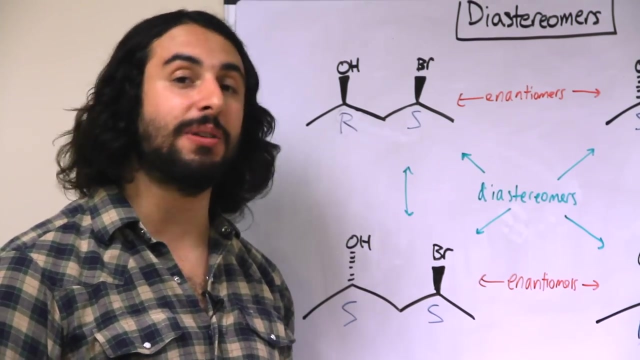 here. if we swap the wedged hydroxyl for a diastereomer, we're going to get a different stereoisomer, because these are not the same molecule. they differ in how they are oriented in three-dimensional space, but they are not specifically mirror images of each other. they do not have a 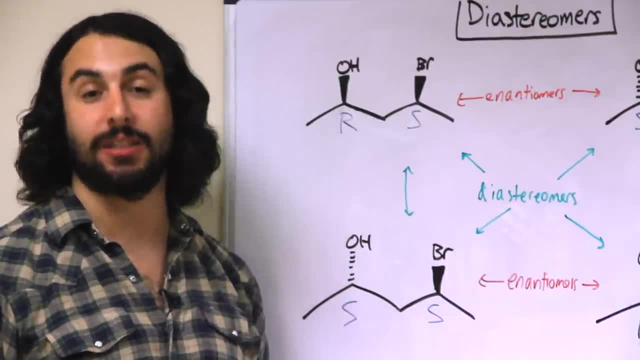 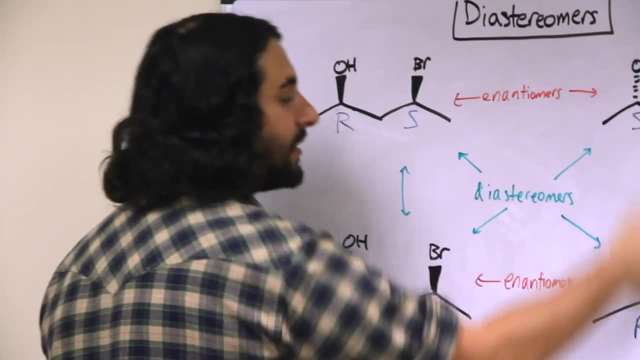 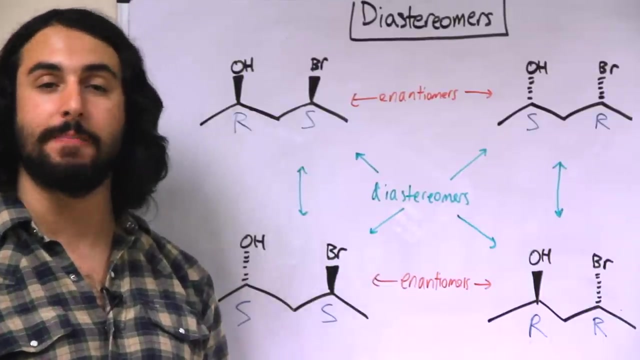 mirror image relationship, so they cannot be enantiomers of one another. so that's what diastereomers are. these are different diastereomeric relationships because they are stereoisomers of one another, but not specifically the mirror image. so basically, what we want to understand is: 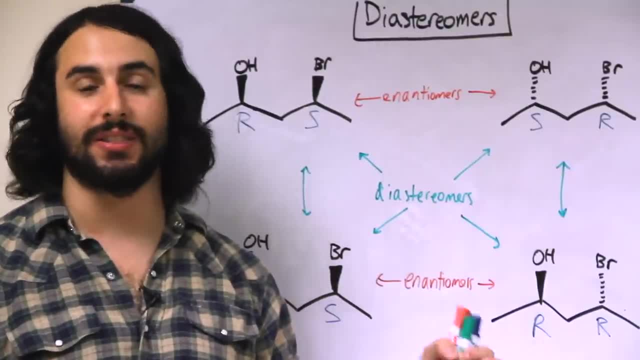 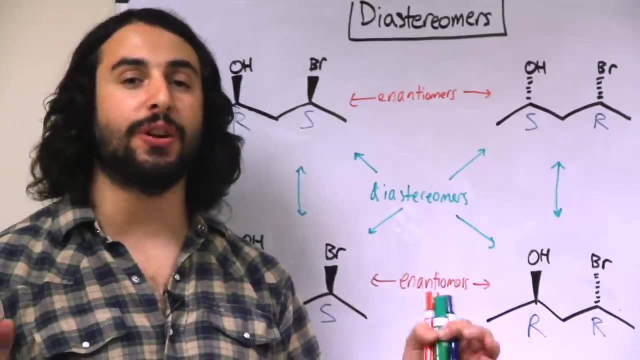 that any molecule, no matter how many stereocenters it has- let's say there's a compound with 10 chiral centers- that means it could have many, many, many different diastereomers, because if you invert only one or two or three or four. 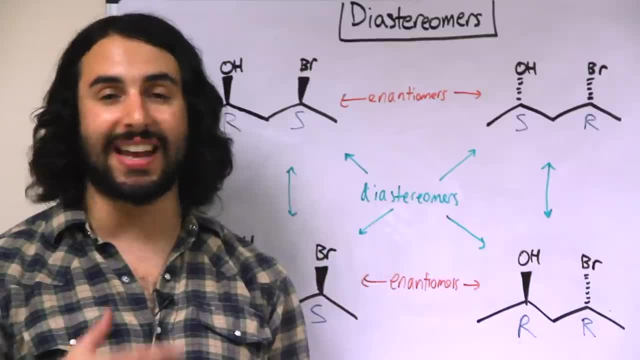 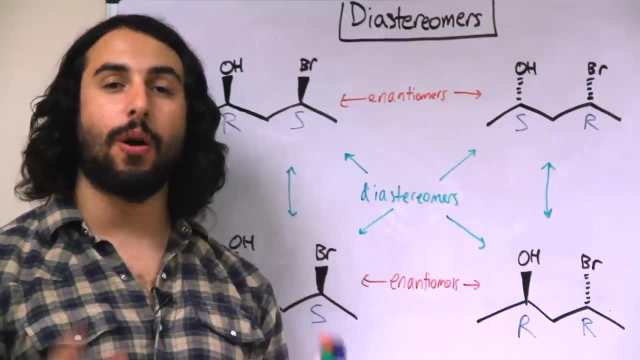 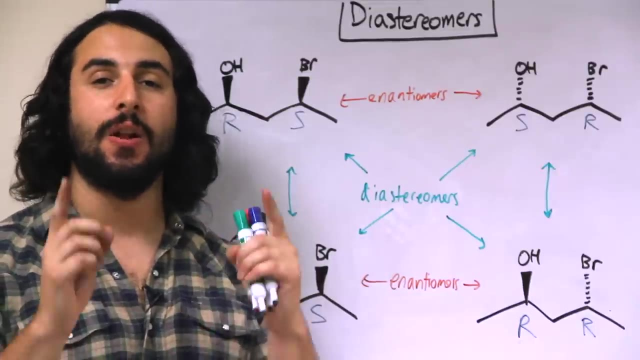 or up to nine of those stereocenters, in any combination you can think of, you would generate a different diastereomer of that molecule. however, there can only be one enantiomer of any given molecule because it is specifically the mirror image of that molecule or the molecule. 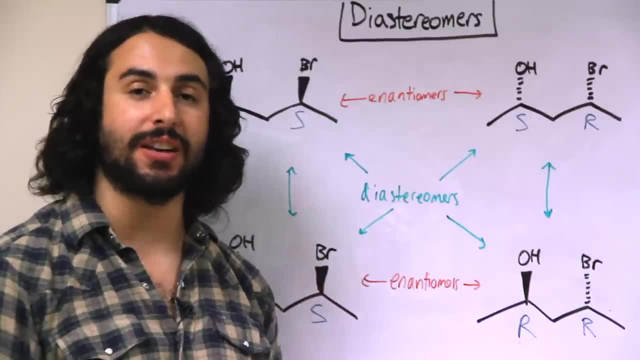 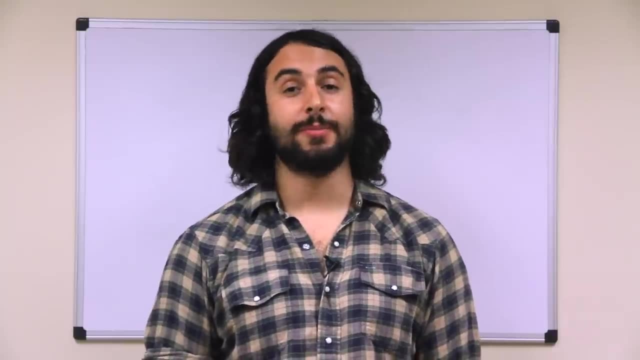 in which every single one of those chiral centers is inverted to the opposite absolute configuration. thanks for watching guys. subscribe to my channel for more tutorials and I'll see you in the next video and, as always, feel free to email me of questions.